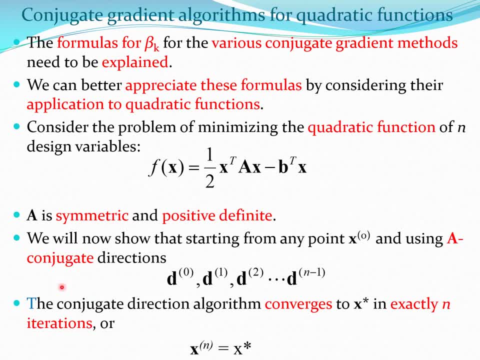 x0 and using a conjugate directions d0,, d1, d2, all the way to dn-1,, the conjugate gradient method will converge to the solution x star, which is the optimal solution of this function f of x, at exactly n equals k or k equals n. So essentially, mathematically speaking, 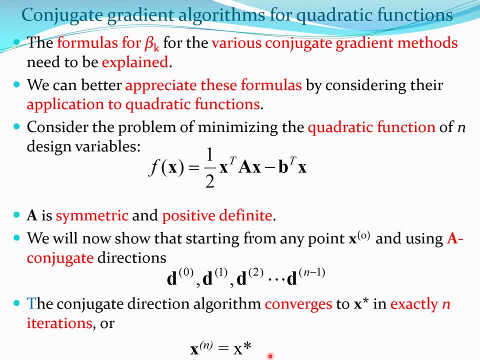 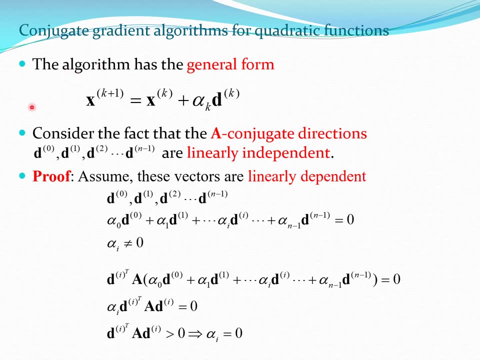 we can say that xn is going to be x star. So this is a fundamental fact that we are going to prove in the next few slides. So, basically, let us go back and start with the general optimization algorithm, which is: xk plus 1 equals xk plus step size into search direction dk. Now we are going to use a fact in this. 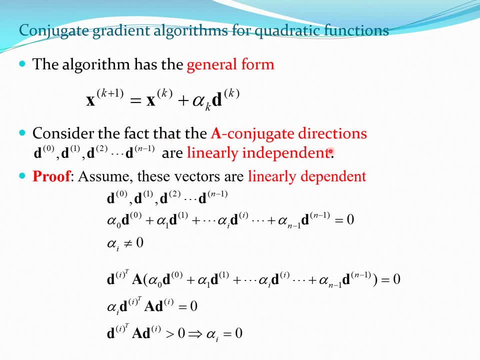 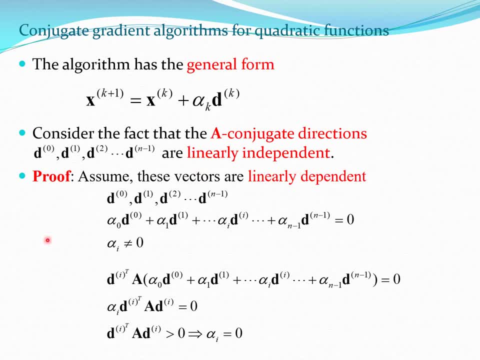 So we can prove this by using a fact in this derivation that these conjugate directions d1, d2, dn-1 are linearly independent. So we can prove this particular fact by contradiction. So let us resume that this is not so and actually these vectors are like: 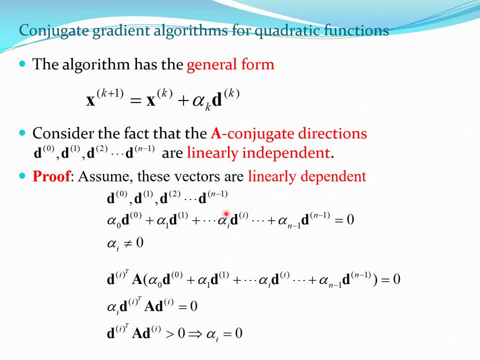 this set of vectors, we can write out a particular equation in this form: α0d0 plus α1d1, all the way to αn-1dn-1, equal to 0. And if, if you, if, if, if vectors are linearly dependent, then certainly one of these values of alpha is not going to be. 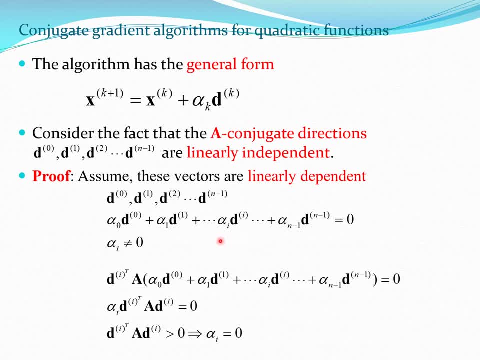 equal to 0.. Okay, so let us assume that is alpha subscript i. Now let us say this is true. then let us go back to the equation here and pre-multiply it by d. i transpose a. So we pre-multiply this equation and essentially what happens is that there is a lot of vanishing and all the terms. 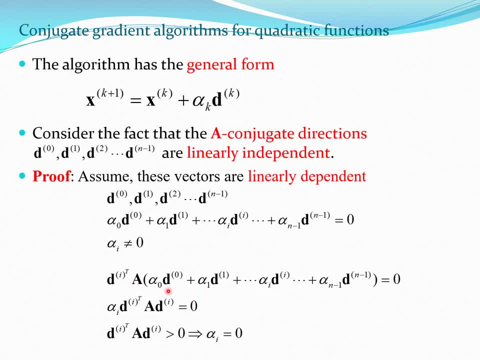 where i is not equal to, i essentially get decimated because of the a conjugacy property, and whatever remains is this term alpha i, d i, t a d i equal to 0.. But we have started with this, thinking that a is positive, definite and therefore 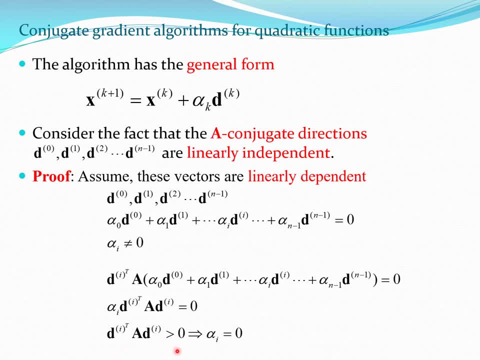 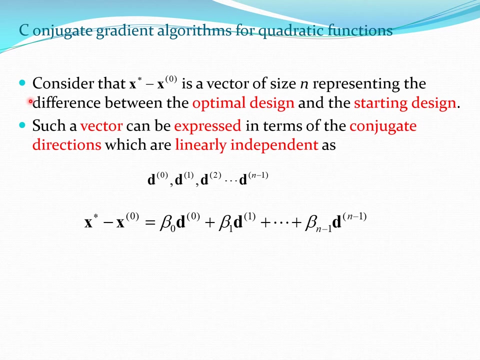 d i, t a, d i is greater than 0. Now, for this to happen, alpha i must be 0, and therefore we have proved by contradiction that the conjugate directions are linearly independent. So we are going to use this property now. and to use this property, let us consider the vector. 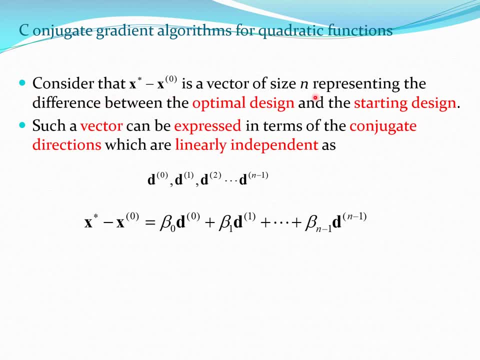 x star minus x 0, which is a vector of size n And represents the difference between the optimal design x star and the starting design x of 0. Now such a vector can be expressed in terms of conjugate gradients in this manner. So, essentially, if this is a vector, i can write it in terms of the conjugate gradients with: 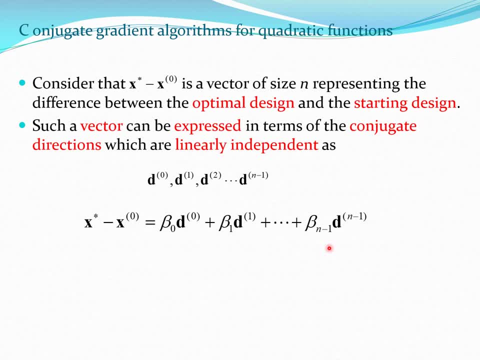 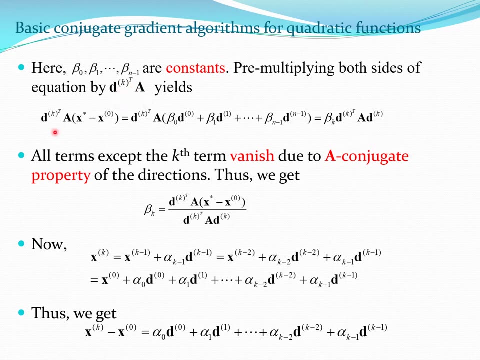 certain constants- beta 0, beta 1 to beta n minus 1, which are general values which we need to calculate. We take that last equation and we pre-multiply it by d, k, t, a. So essentially we get this equation here and what happens is that, again because of this, a conjugacy property, lot of the terms. 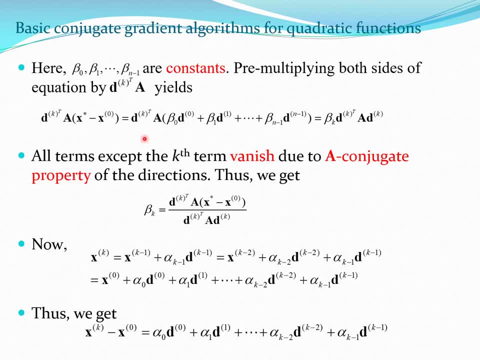 vanish on this side, and all the terms where d superscript k is not present will become 0, and so finally, you are going to get the term beta k. So this is the only term which is going to survive and therefore I can get an expression. 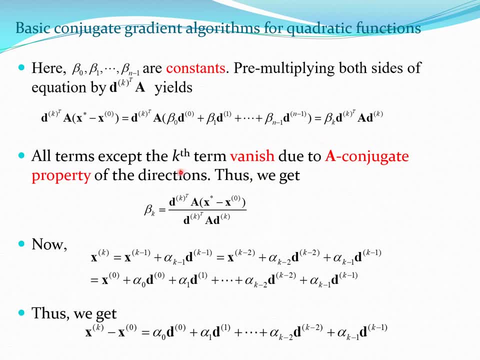 for these beta values which is given here. beta k is this: d k, t, a, x star minus x, 0 by d k, t a d k. Now we are going to spend some time trying to further simplify this definition of beta k here. So let us look at x k. 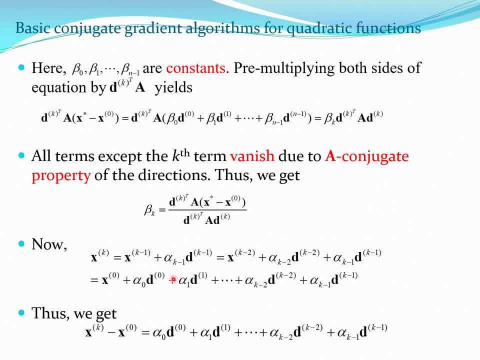 Now x k is going to be x k minus 1 plus alpha k minus 1 into d k minus 1, which is the general search formula. Now you keep going backward in time, so this will then become x k minus 2 plus this term. 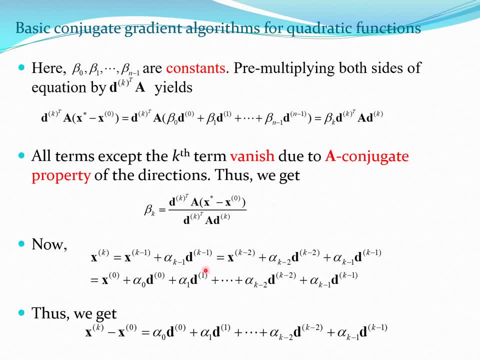 here with k minus 2 and this term here. So all we are doing is we are expanding this whole thing out all the way to x of 0. So if you do that, you get this equation here: x k is x 0 plus alpha 0, d 0.. 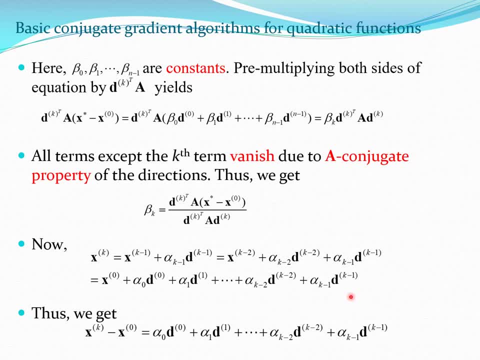 So alpha 1- d 1, all the way to alpha k minus 1, d k minus 1, and therefore I can then write x k minus x 0. is this equation here? so essentially, this is coming out of this here. Now I essentially have two sets of equation. one is x k minus x 0 and the second is x star. 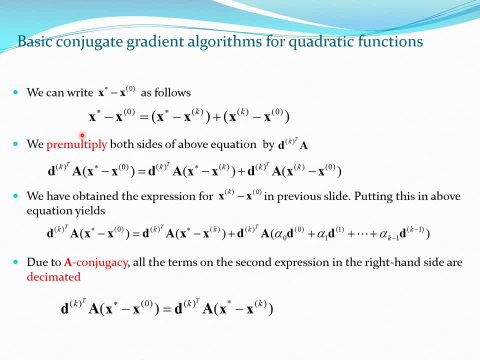 minus x 0, and we are going to use these two equations next: So x star minus x 0.. So x star minus x 0.. be written as x star minus x k plus x k minus x 0, because x k would cancel out. so we pre-multiply. 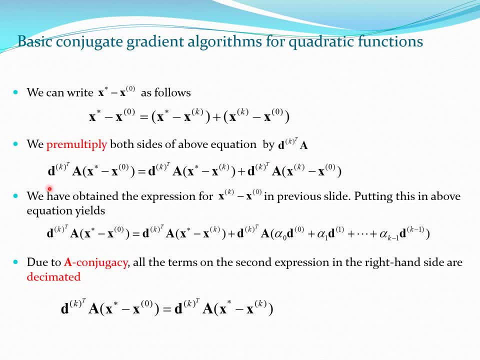 both sides of this equation by d, k, t, a, and we get this equation here. now we have obtained the equation for x k minus x 0 in the previous slide, so substitute that equation here and we get this big term here with all the terms ranging from alpha 0 to alpha k minus 1. now, once again, you 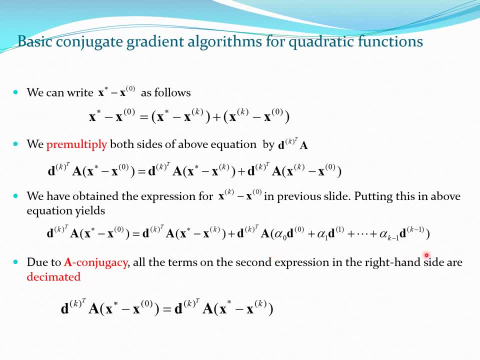 think about the a conjugacy property. all these terms do not have k in them and therefore they are all going to be decimated or wiped out and essentially whatever is going to be left is this term here and this term here. so two terms are going to survive this process and these are the 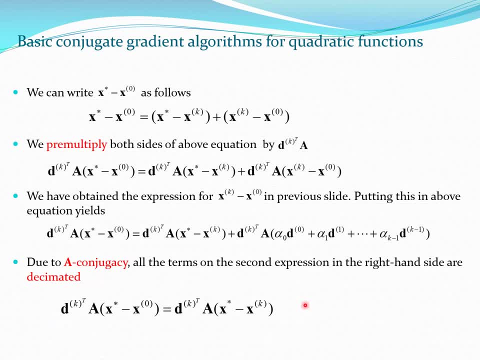 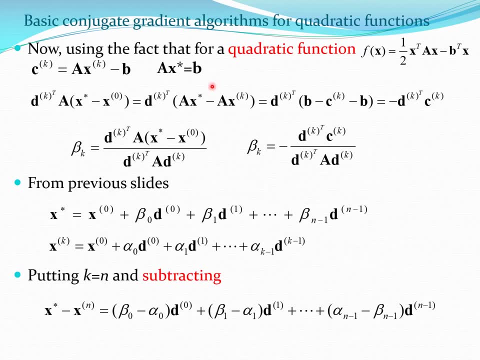 two terms here. okay, so you can take a look at this. now we are going to further simplify this equation here. to do that, we go back to our quadratic function and we realize that if we were to differentiate this quadratic function and get the gradient, we would get c, k is a, x, k minus b from direct. 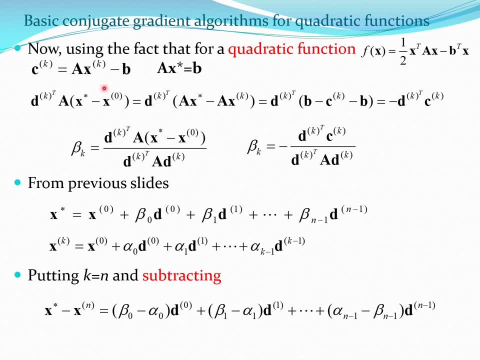 differentiation, and also at the optimal point this gradient would be zero. so if we set a x k minus b to zero, we get a. x star is b, where x star is the optimal solution. therefore i can write this last equation like this, where i have brought the a from outside to inside here: 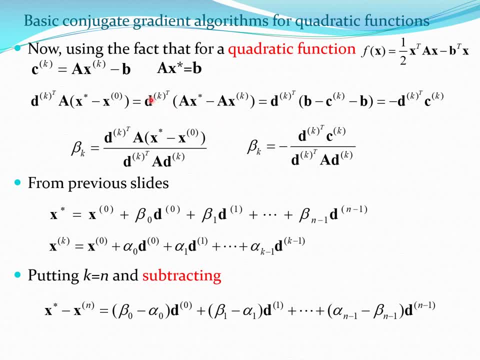 so it has become a x star minus a x k, and then i use a x star is b. from here i use a x k is c k plus b, and i put that here. there is a cancellation of these two b's and i get minus dk. 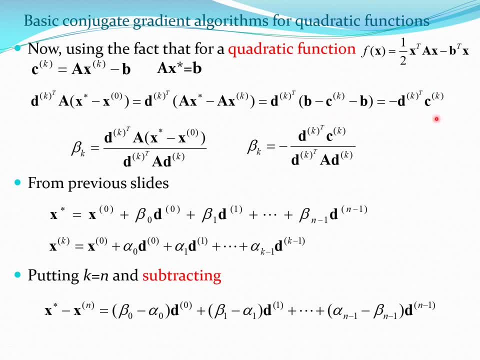 dkt ck. So this is nice compact expression and by looking at this expression and this expression here I can simplify the whole problem here. So I can get beta k equals dkta x, star minus x0 by dkta dk. So this was in the previous slide and so if I take this term here now and I 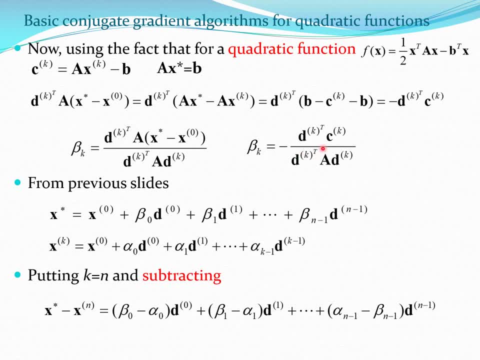 realize this is minus dkt ck. the numerator becomes like this and I get this compact expression. So this is the expression for beta k which I have obtained. Now again, go back to our previous slides and recall that x, dkta, x star minus x0 by dkta dk. So this was in the previous slide and so if I take this term here now and I 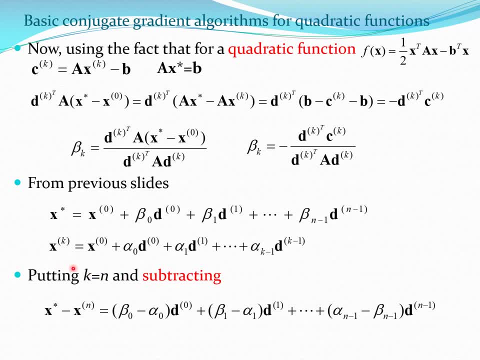 was this series here and xk was this series here. Okay, so in x star we had beta 0 terms, beta 1 beta terms, and so on. in xk we had the alpha terms, and here we had d0 to n minus 1, here we had d0 to k. 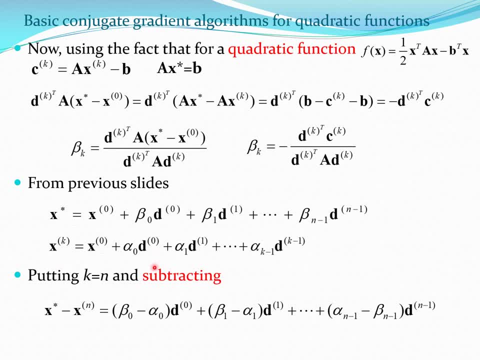 minus 1.. So now what we do? we put k equals to n in the second equation and we subtract these two equations So we get x. star minus xn is going to be this series here. So now we are going to look at this particular series and we are going to realize that if 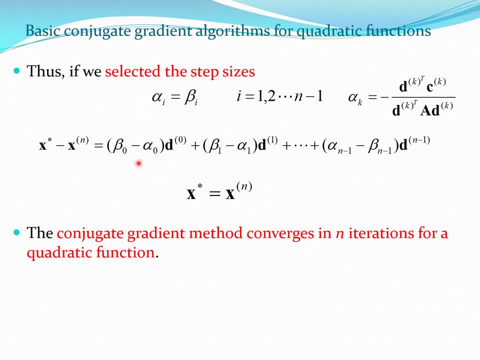 alpha i and beta i are same, then all these terms are going to be 0 and therefore x star is going to be xn. Therefore, all I have to do is select: alpha k is beta k or alpha k is minus dkt, ck, dkt, adk. and if I were to do that, the conjugate gradient method would converge in exactly n. 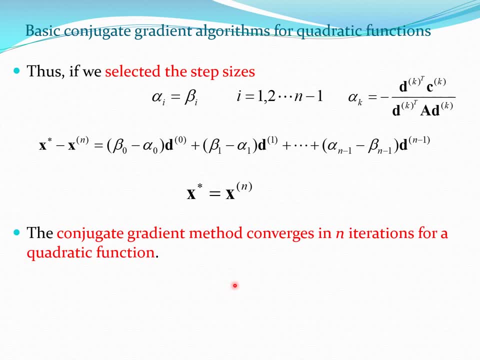 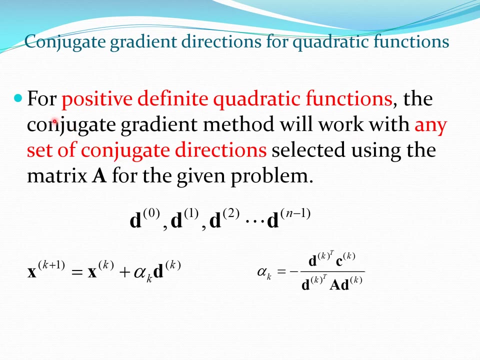 iterations for a quadratic function. So essentially, this is something we have been saying for a long time. Now we have proved it and also we have found the step size value here as a closed form solution. So let us summarize what we have done till now. What we have seen is that for a positive, definite 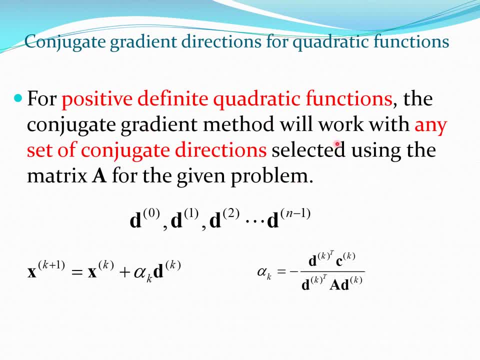 quadratic function. we have to have a positive, definite quadratic function. So we have to have a positive, definite derivative function. The conjugate gradient method will work with whatever set of conjugate directions you can get using the matrix A. So let us say you use the matrix A to get these. 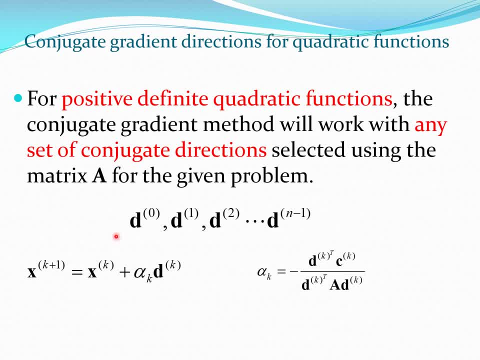 conjugate directions, and then you just have to use the general algorithm and you also have the step size value and then you are going to work out with your algorithm. Now, just in a few slides, we are going to actually address the issues of how do you get these. 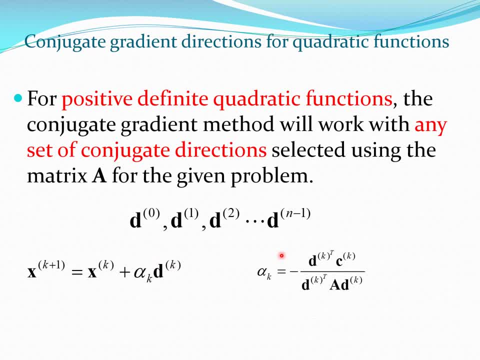 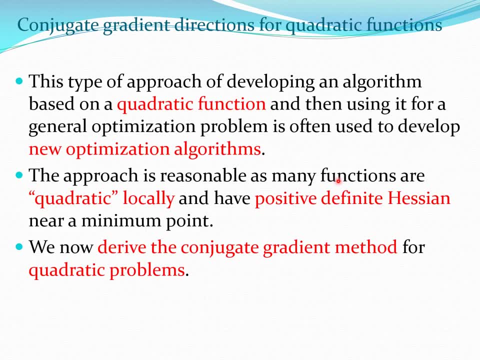 certificate vectors taking different search directions, and which ones are different from the solved ones. And so let us say, for example, we have tried to do this without right say correcting or Ish Taste with an earthquake start method of the symmetric tweet method, or mezzanine renders with a juntic. 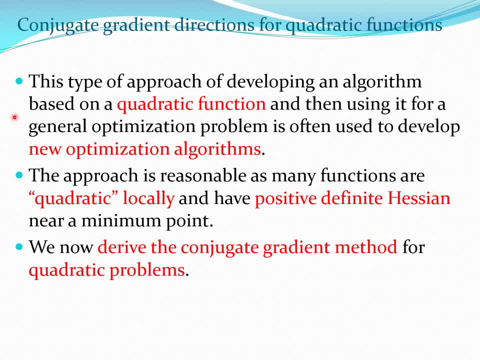 מע 1959 " mezzanine renders, mezzanine mezzanine quantam. mezzanine mezzanine mezzanine Fighter, mezzanine mezzanine bender. because many functions are quadratic in a local sense and have positive, definite Hessian matrices. 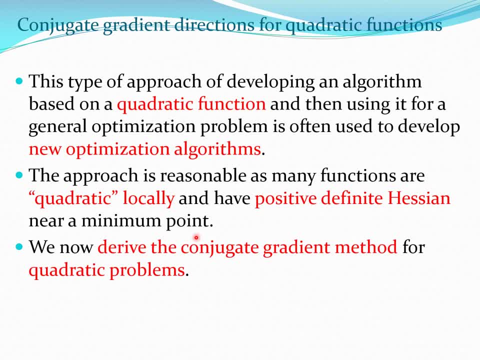 near a minimum point, which is the approximation we are making here. We are always presuming that the matrix A for the quadratic form is a positive, definite matrix. Now we are going to look at the conjugate gradient method for the quadratic functions. So let us again go back to our 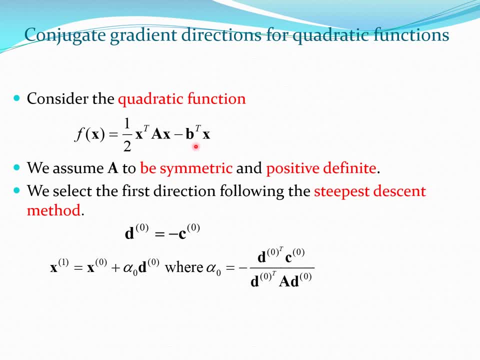 quadratic function f of x, half x, t, A x minus b t x. And again we assume that A is symmetric and positive definite. Now the first search direction comes directly from the steepest descent method. So d 0 is minus c 0.. We already know how to go to the next point: x 1.. x 1 is going. 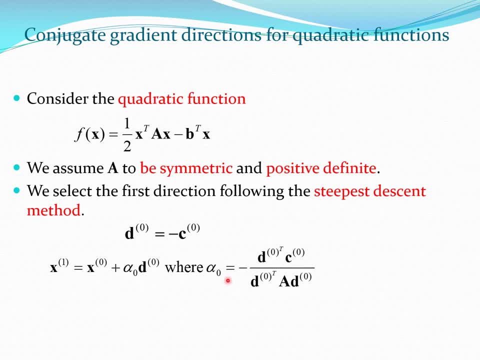 to be x 0 plus alpha 0, d 0.. And for alpha 0, we have already derived this particular function Equation. So if we have A, we have d 0, from here We have c 0.. We can quickly calculate this. 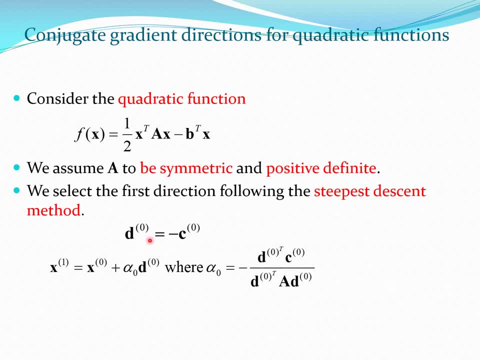 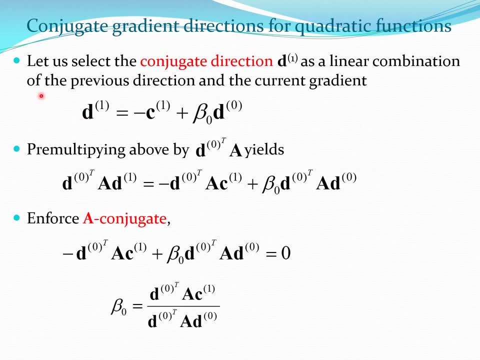 particular value. So that gives us the starting value of d 0.. But now we have to calculate d 1,, d 2 and so on. So that's what we'll do next. So let us say, we now look at the next conjugate. 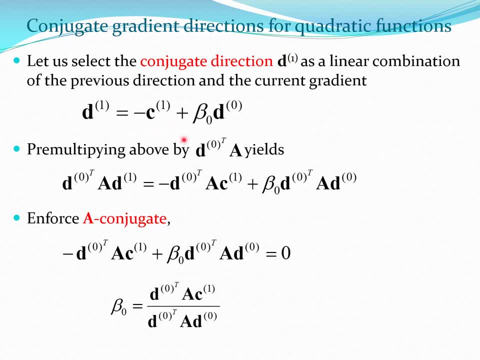 direction d 1.. So d 1 is going to be minus c 1, plus some beta 0, d 0, where we still don't know the beta 0.. Now pre-multiply both sides of this equation By d 0, t, A, which we do here, And as soon as you do this, you can realize that you have 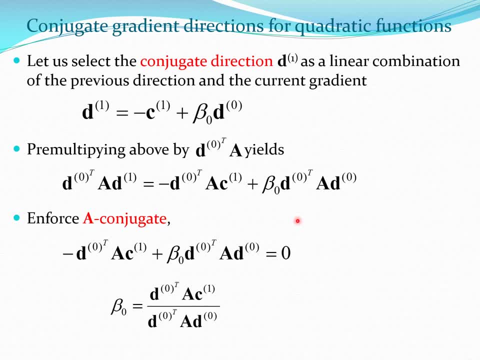 a particular term where you can use this conjugacy factor. Okay, And essentially this is the term. because d, 0, t, A, d, 1 must be 0, because 0 and 1 are different, So this entire term becomes 0.. And you write this term as 0 here And this immediately gives you your solution. 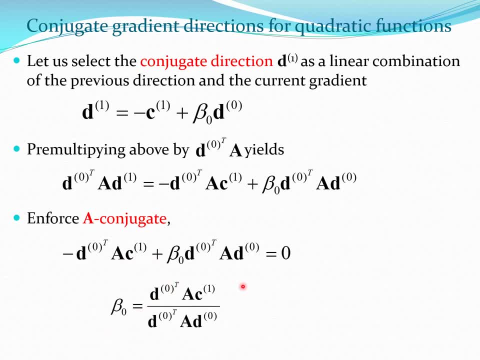 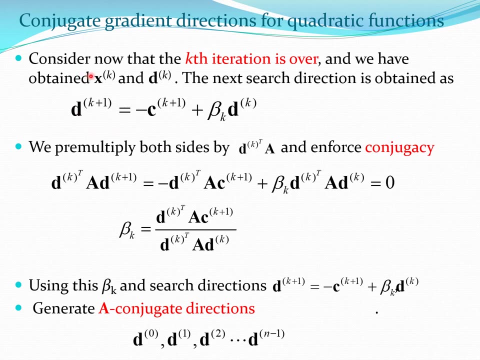 for beta 0. So that essentially gives you the first value of beta 0 here, And with that you can calculate the direction d 1.. Now extrapolate this to the kth situation. So let us say you are at the k. 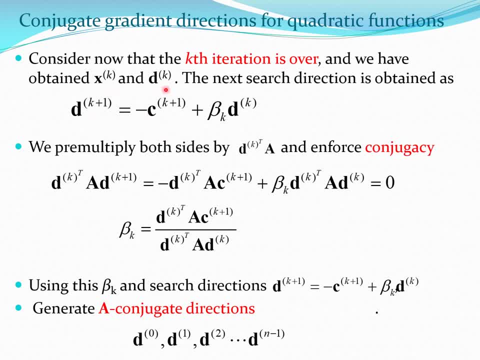 plus 1th point, and you have obtained x k and d k. So the next search direction is going to be: d k plus 1 is minus c k plus 1 plus beta k into d k. Now pre-multiply both these sides by d k, t A, which we have done here, And again enforce conjugacy which: 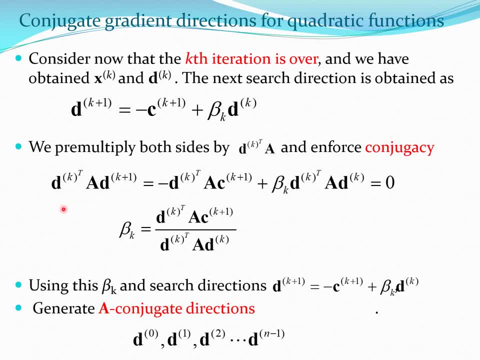 means that d k, t A, d k plus 1 must be 0, because d? k and d k plus 1 are A conjugate And therefore this equation must be 0.. Now, once this equation is 0, I can get beta k in this form. So essentially, 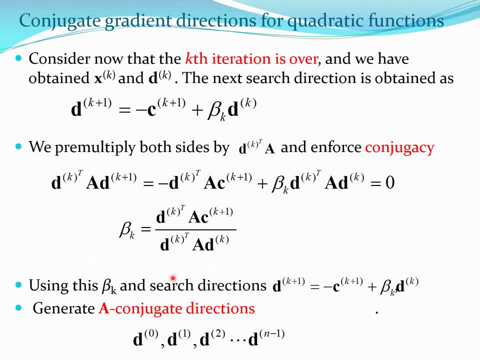 whatever we did in the previous slide, we now generalized it to the kth point, So essentially at every point we can now generate a search direction using this general formula. here Now use this beta k and the search direction d k plus. 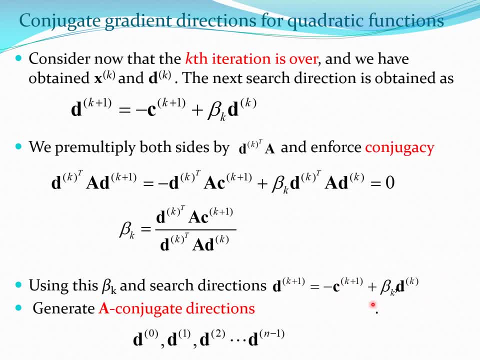 1.. You get this value here. You have minus c k plus 1, plus beta k into d k. Generate all these conjugate directions: d 0, d 1, d 2 to d n minus 1.. And you can then solve the problem. Now, if you, 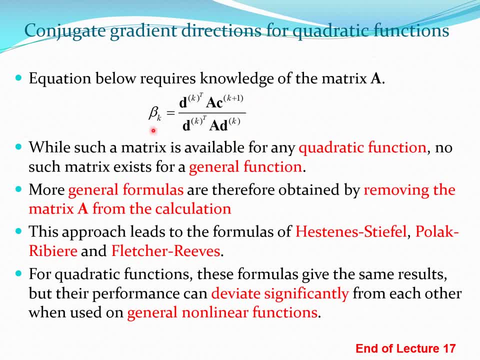 look at the beta k values which we have derived, we see that this beta k would require a search function which would require you to know the value of A. And this method, of course, can be used if you have a quadratic function, because if you have a quadratic function you would have a value. 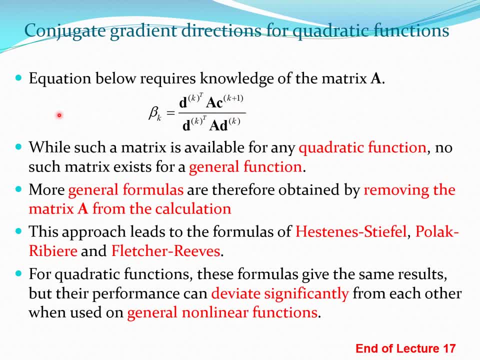 of A, And you can also obtain the value of c, k at any point. Now, what we are going to do next, in the next lecture, is you are going to generalize this formula such that A is no longer there. We are going to get rid of this A matrix from this formula. But again coming back to this formula, 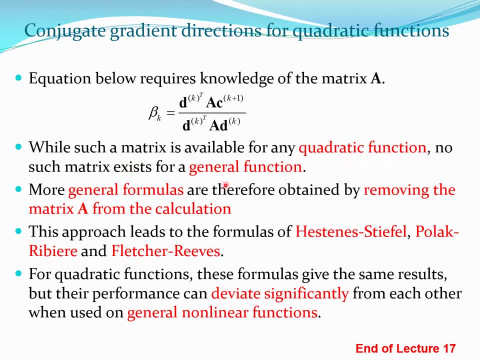 we see that such a matrix is there for all quadratic functions, but we won't have it for any general function. So in a general formula we try to remove this matrix A from certain derivations and calculations. And that is what actually Heston, Stifel, Pollack, Rebier and Fletcher-Reeves 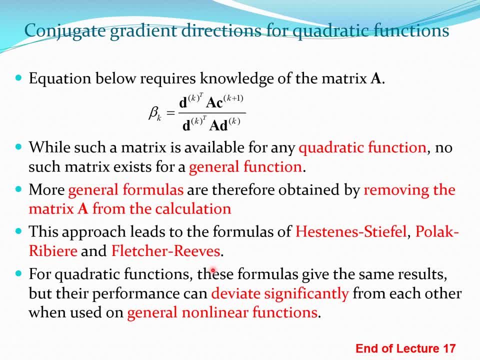 have done, And they have given us these nice formulas which we have looked at, which are expressed only in terms of the search directions and the gradients, So no A matrix comes there, though these formulas are actually derived from a situation where you are presuming a quadratic function, So 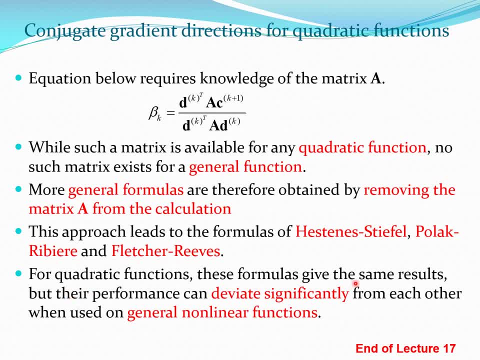 that is something which is interesting. Now for quadratic functions. all these formulas will give the same results, but their performance can deviate significantly when you apply them to general nonlinear functions. So essentially, this video was a somewhat deeper and more mathematical study. 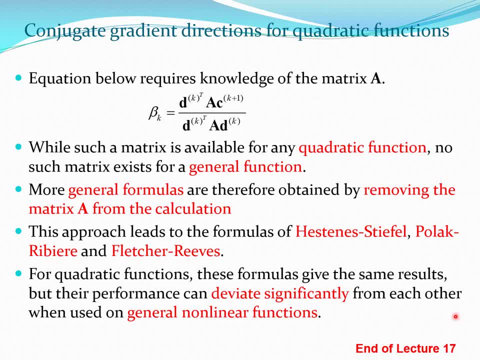 of the conjugate gradient method and how some of the formulas which are used in the conjugate gradient methods can be derived, because in many books you will find that the conjugate gradient methods and many methods are presented straight away without any particular proof or any derivation. 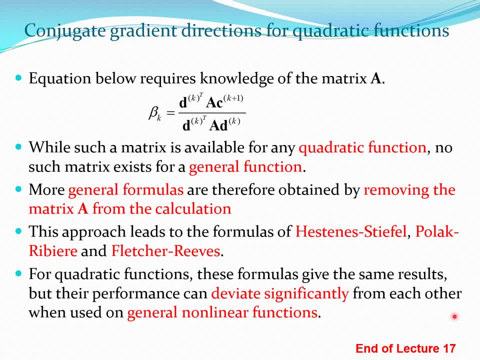 So very often, students are using these methods as tools, without understanding the genesis of these methods, which is very important to understand the strengths and weaknesses of these methods. If you are learning more about the stoichiometry of junto science, you can find out that there is: a sample method where you can use this method as a tool whatsoever. The Execution Centre provides a sample method that is a fun. another example of the methods that are used for all Heston and Stifel. I am not going to put my second study, okay, here. 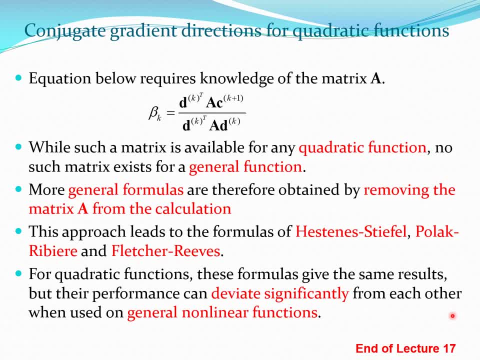 Instead of the drop talk, for example, what it is an exercise users are going to do, except for the study of the two conjuguate gradient methods, As you remember, weaknesses of these methods and also, in case you ever want to create new algorithms or even read, 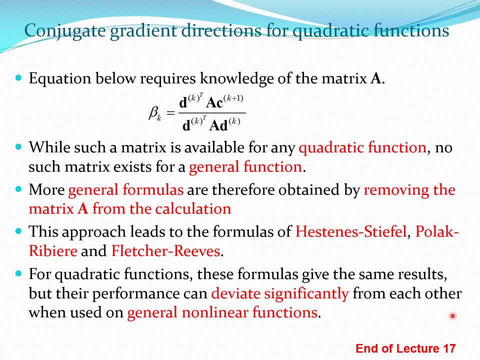 the literature. it's interesting to know some of the genesis of these conjugate gradient methods, because they are very powerful methods and are used in optimization for very large degree of freedom systems. So I'll stop this lecture here and we will meet again in the next video, where 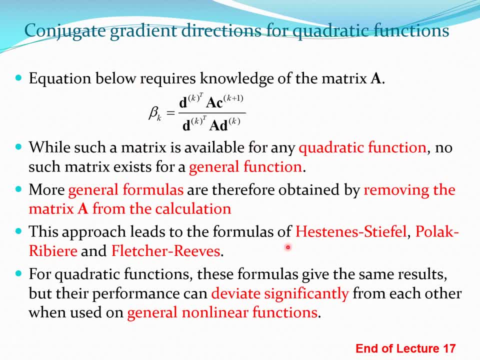 we are going to use this particular beta k to derive expressions for the Heston, Stifel, Pollock-Rabier and the Fletcherese method. Thank you very much for listening to my video and please subscribe to my channel and inform different people about this particular set of lectures. 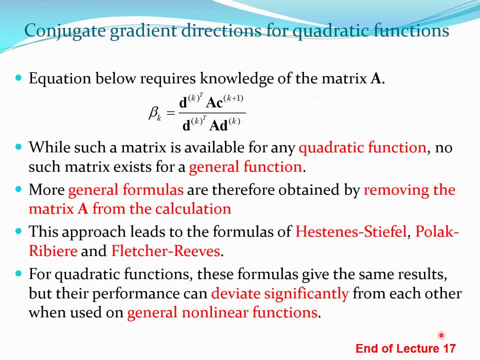 which I have posted here. If you want to look at some examples on this particular topic, you can consult my book, which has a plethora of examples on how to get conjugate directions and so on. Thank you very much. Thank you.